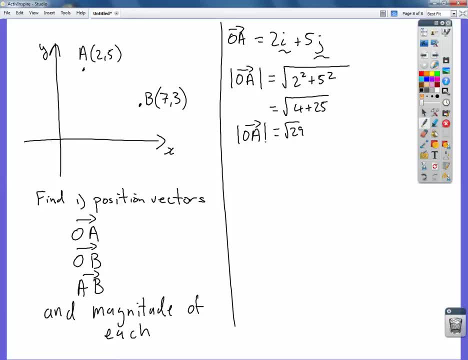 it like that rather than. I can't make that any simpler. Same again now for OB. OB, it goes from the origin to B is 7I plus 3J, and the magnitude from O to B is 7 squared plus 3 squared, so 49 plus 9. 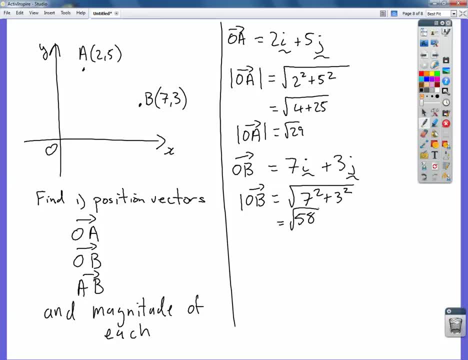 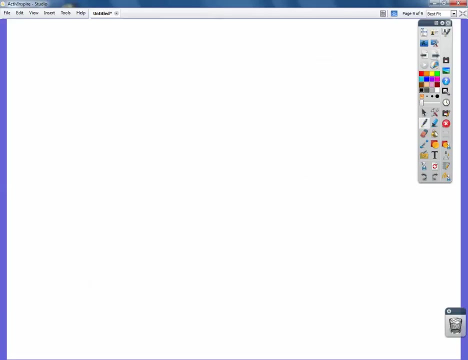 gives me 58, the square root of 58. And I won't worry too much about that. Now we want the vector from A to B. From A to B, So from A to B. I'm just going to have to go onto the new page We've got. 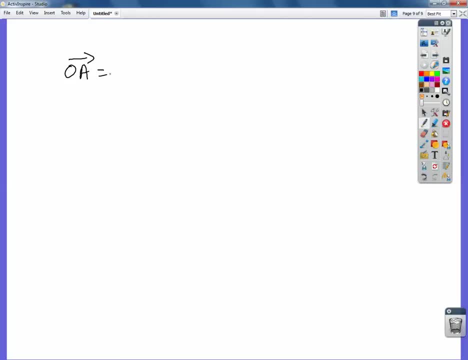 OA we said was 2I plus 5J. OB is 7I plus 3J. Now think about this: Here's OA, here's OB. we want that one there from A to B. So you'd notice that I can add that. 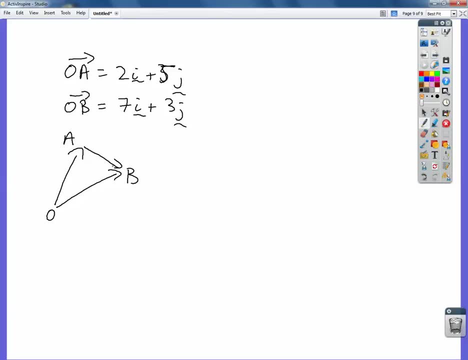 OA plus AB is going to give me, if I look at that triangle, the vector from OA plus the vector from AB. when I add them together is going to give me the vector OB. I want AB by itself. so that's going to be the OB minus OA, which essentially is the same as what we've done before: final minus initial.